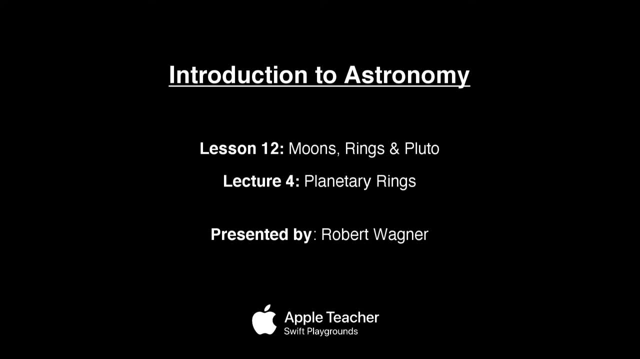 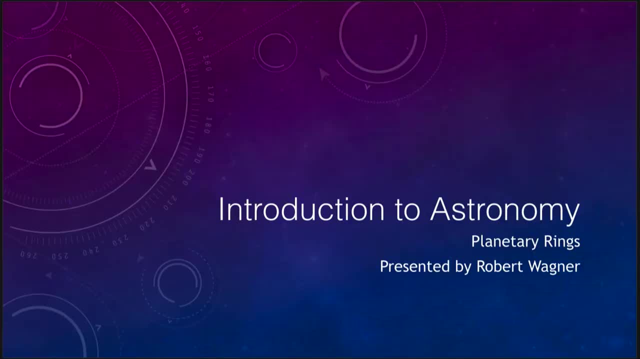 Greetings and welcome to the Introduction to Astronomy. In this lecture, we are going to talk about planetary rings, or rings that exist in the solar system. Now, the best known of those are around Saturn, but there are a number of planets that have rings as well, So let's take a look at what we see here. 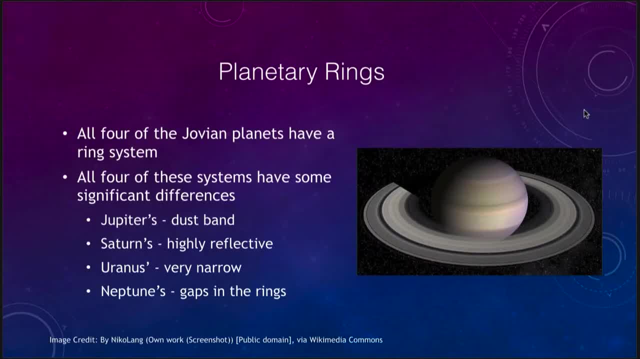 And we look. first of all, here's our image. This is the planet Saturn and you can see its ring system stretching out around it, But it is not the only planet with a ring system and in fact, all four of the Jovian planets will have a ring system around them. 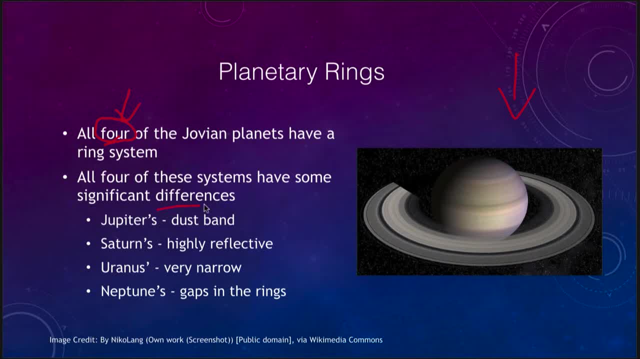 However, there are differences between each of these. Saturn's is highly reflective and prominent, very easy to see and we can see that here in this image. And in fact, Saturn's were the first rings to be detected. The next set to be detected were those of Uranus. 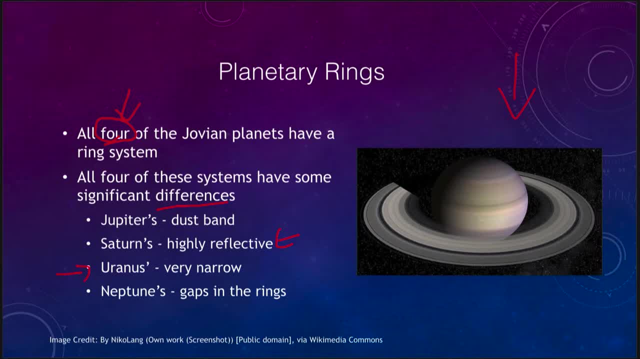 Uranus has very narrow rings and very dark rings, And they were detected when a star was occulted by the rings, or the rings blocked out the light of that star and caused it to dim. Jupiter's were the next detected, which are a very faint dust band, some very minor rings. 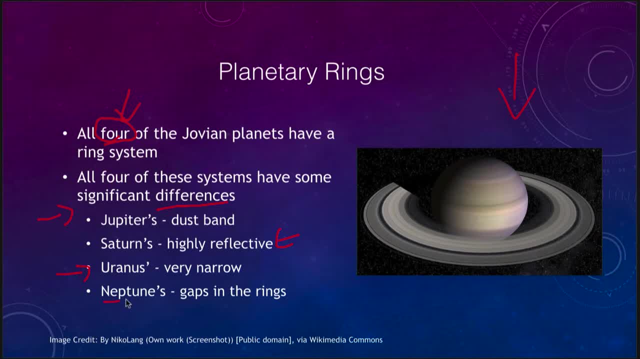 But there is at least some portion of a ring, And Neptune's are unusual in that there are gaps in the rings, So they are not nice smooth rings here, but there are actually areas where the material is denser and areas where material is less dense. 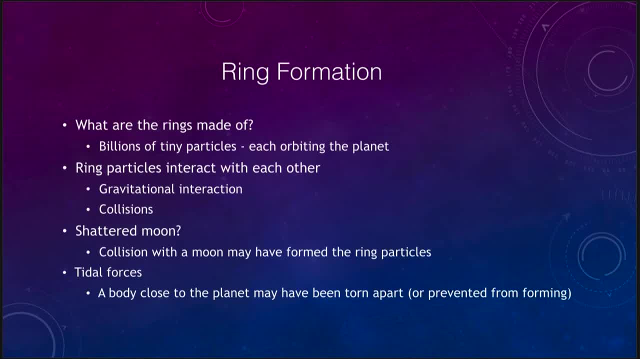 So let's look at ring formation. Where do rings come from in the first place? Well, first of all, what are the rings made up of? They are billions of tiny particles each orbiting the planet. You can think of them each as a small moon. 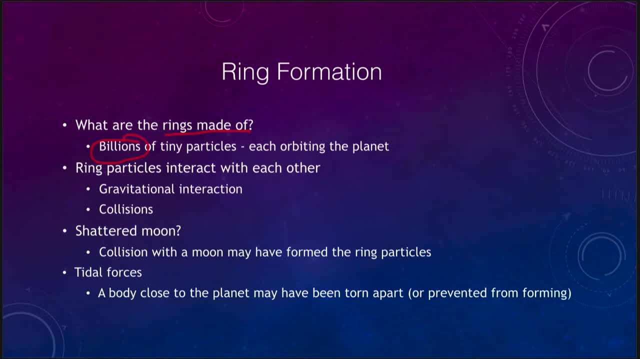 So there is a small moon orbiting each planet, and each of these is very small objects. They may only be a few centimeters in size, They may be up to a meter or so in size, But they are not gigantic objects by any sense. 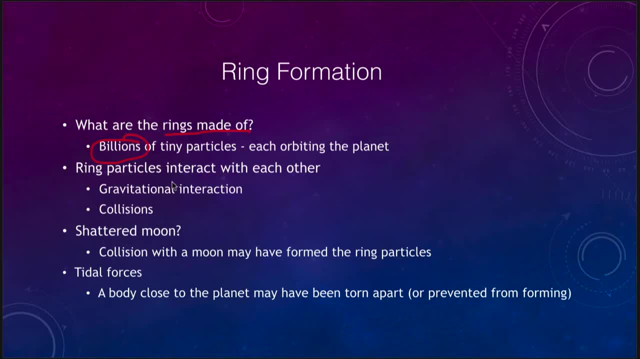 The ring particles do interact with each other, by gravity, which keeps them together, and through collisions. So the particles will collide together as they orbit and that will give us the structures that we will see Within the rings. Could these be a shattered moon? A collision with the moon might have formed the ring particles. 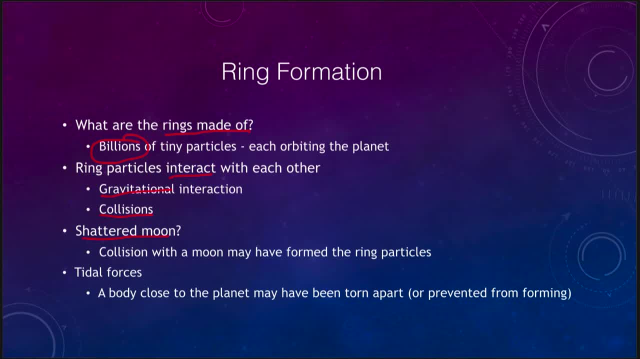 So if a large object crashed into a moon and recall that these Jovian planets all have lots of moons, That could have expelled a lot of ring particles out into space that could have been captured in a ring. So perhaps some sort of collision with the moon or tidal forces as well. 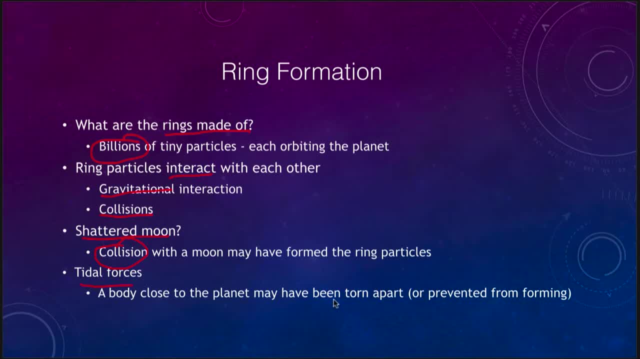 An object that gets close enough to the planet Could have been torn apart by its tidal forces, The gravity on one side of the object, the near side, being stronger than the gravity on the far side, Because the gravitational force depends on distance. 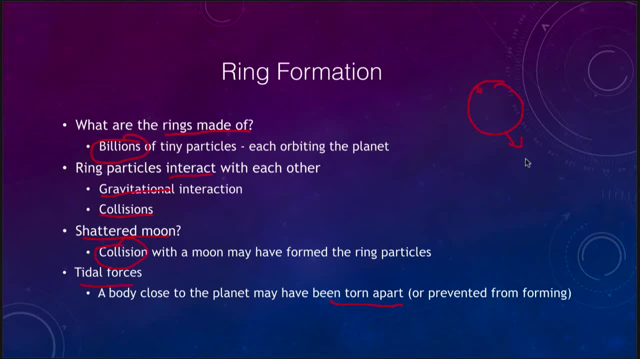 If you're close enough to the object, it's quite possible that the object will not be able to hold up structurally to a significant force on one side and a very small force on the other. Essentially, you're stretching the object apart And in case, if particles are just that close, it may just have been prevented from forming in the first place. 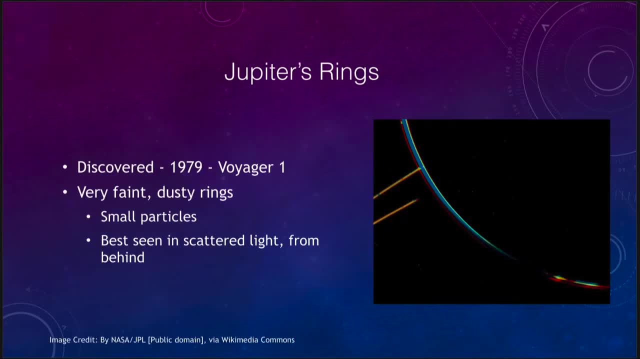 So let's look at the rings of each of these planets. So starting off here with Jupiter's rings, which were discovered in 1979 by the Voyager 1 spacecraft. They are very faint and dusty rings, made up of lots of small particles, And are best seen in scattered light from behind. 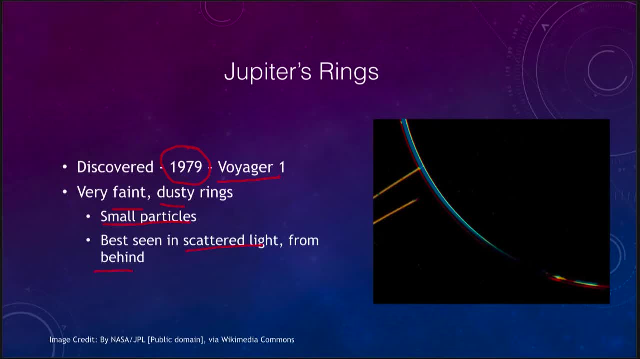 So we don't see them well from Earth Because they're not reflecting a lot of the light, But they do scatter the light through, And if we look from behind Jupiter, as seen by the Voyager 1 craft, We can see the dark, unilluminated side of Jupiter. here. 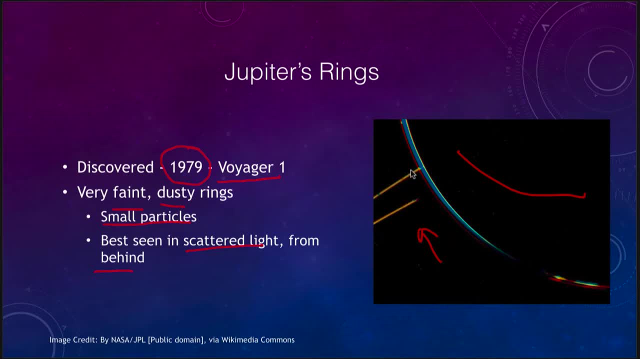 And then we're looking through towards the sun And we can see the very thin illuminated ring, part right here, Going around Jupiter. So Jupiter does have this very faint ring, But not a lot of detail there to learn about. So what we really want to look at are the rings of Saturn. 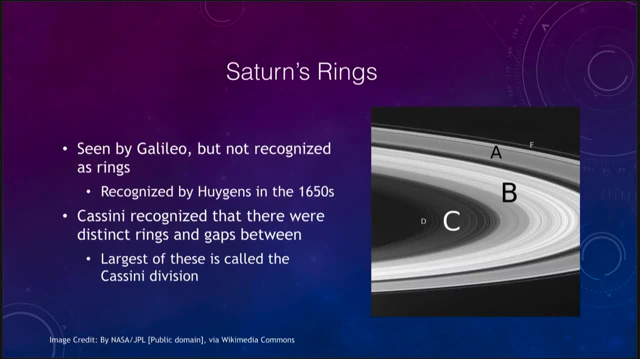 Rings of Saturn have a lot more detail to them, And we can see some of that here. They were actually seen by Galileo, But not recognized as rings, only as a blob on each side of the planet that sometimes disappeared By the time. telescopes got a little bit bigger just a few decades later, in the 1650s. 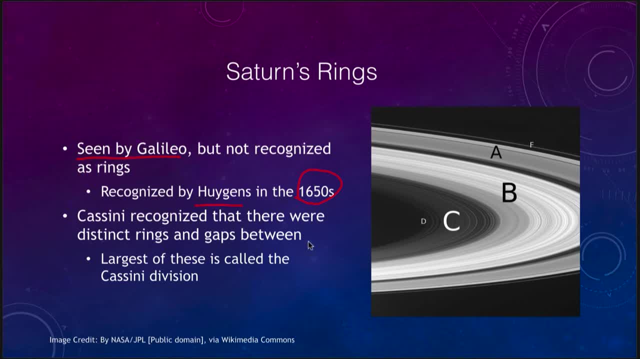 Huygens was able to recognize them as a ring system And around that time, or a little bit later, Cassini recognized that there were distinct rings, Not just a single ring, And gaps between them, So gaps in between the rings. The largest of these is now named the Cassini division in his honor. 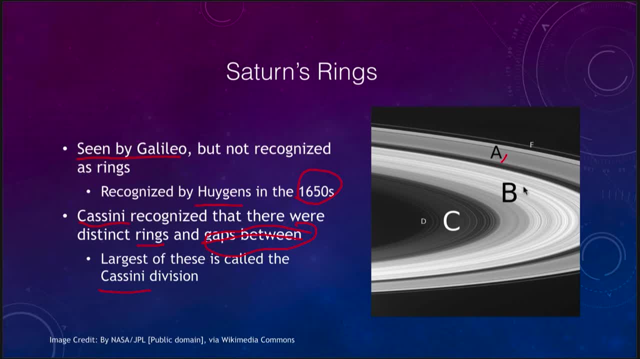 So here we see the A, B, C, D and F rings out here. Primary ones, visible that you'll see, are the A, B and C. D ring is a lot fainter and harder to see. F ring is a very thin ring out beyond the A ring. 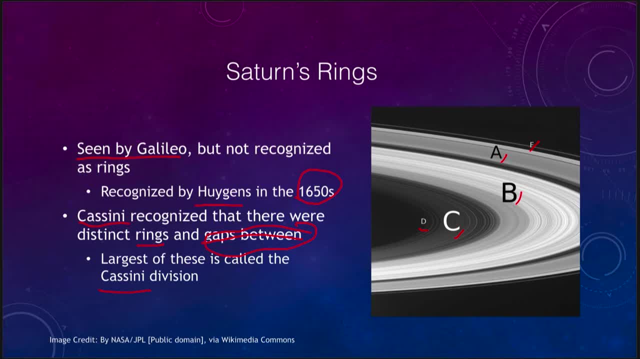 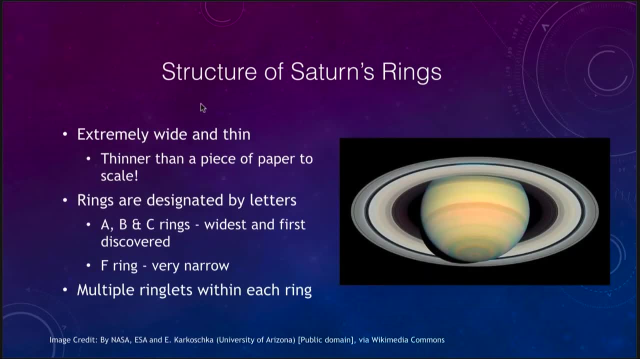 And also a little bit harder to see. So when we look at the structures of these rings, We see, We see that they are extremely wide and thin. In fact, they are thinner than a piece of paper if you took them to scale. So if you scaled them down to a size of paper, 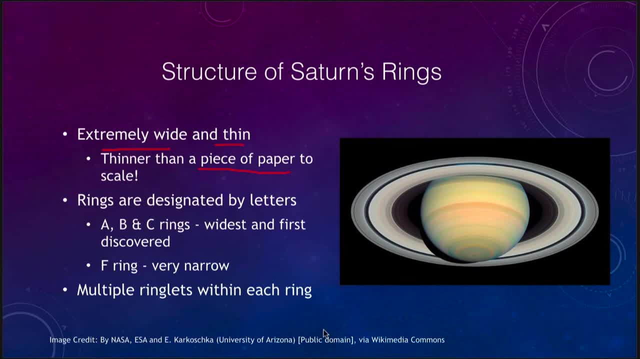 They would be incredibly thin, Much, much thinner than that piece of paper. We designate the rings by letters. They are the primary ones, The A, B and C rings, The first three to be discovered, And those are the primary, widest rings that we see. 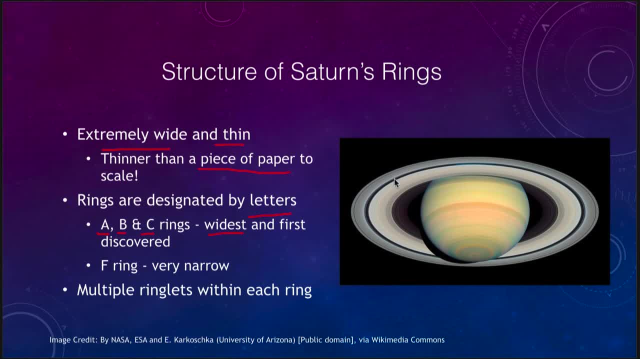 And those are the big bright ones there. And you also have the Cassini division, The gap in between those rings too. So there are gaps, And not just the one, Not just the Cassini division, But you can see that there is another one out here. 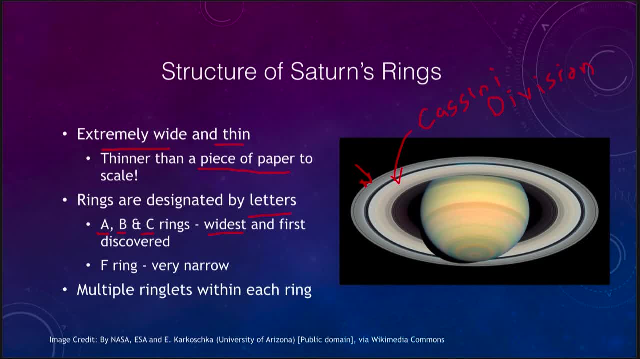 And there are other gaps and structures within the rings as well. So the rings are not just a single ring But actually have multiple ringlets within each ring. And if we look a little bit closer here, Zoom in on the rings, essentially We can see that there are all kinds of structures here. 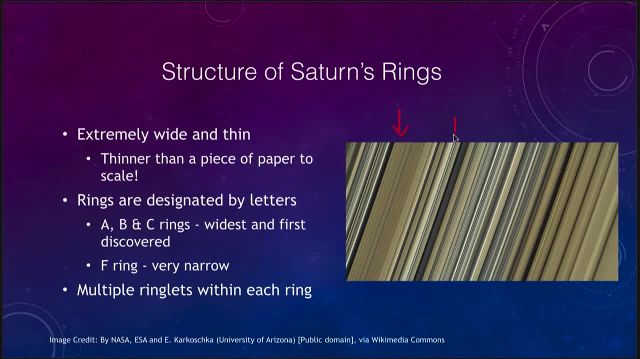 Little gaps And areas where there are a lot more particles, Brighter areas, So big detail Towards what the rings are. There's a lot of structures there And when you think about, within, each of these Are just billions of particles. 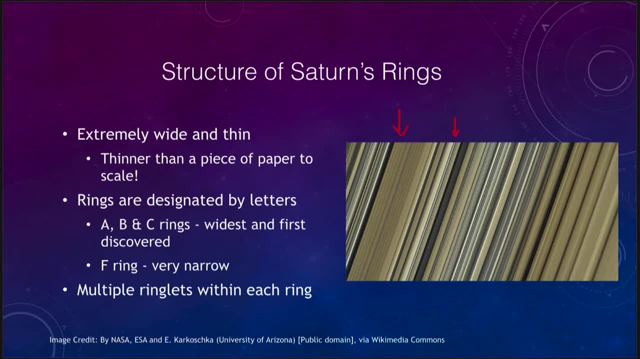 All orbiting around Saturn And kept there. So why do they have this detailed structure? We'll come back and look at that shortly. So let's look here at the compositions. What are these made up of? Saturn's rings are primarily water, ice. 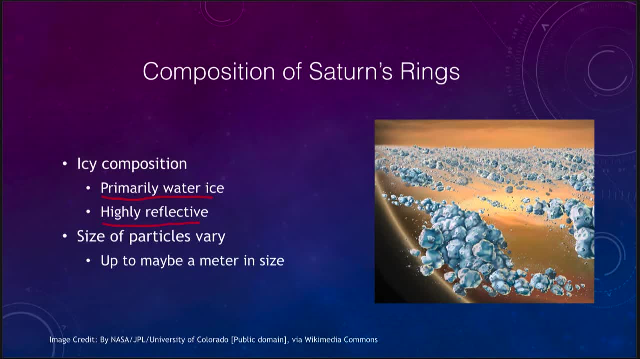 Which makes them highly reflective. So why do we see them prominently from Earth? Because they're reflecting a lot of light. The size of the particles varies, Maybe up to about a meter in size, And some of them will clump together. Now, this is an artist's conception of what the rings might look like. 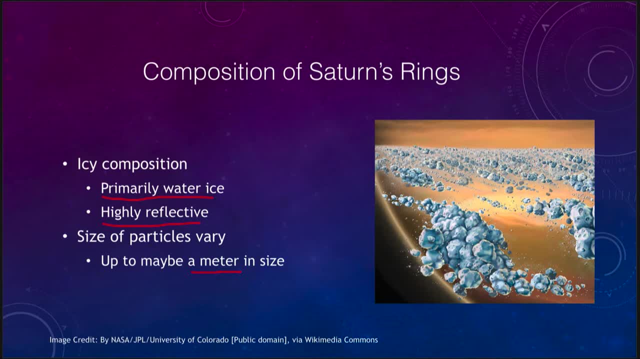 If you were sitting there, inside the rings of Saturn themselves, So you'd have clumps of material And these would likely stick together. They're not strong enough to really hold themselves together gravitationally, So as objects collide They would stick together. 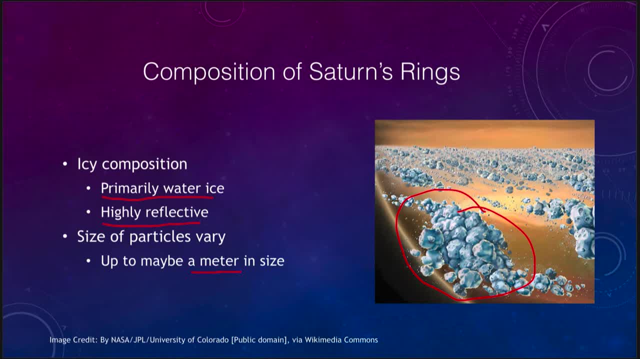 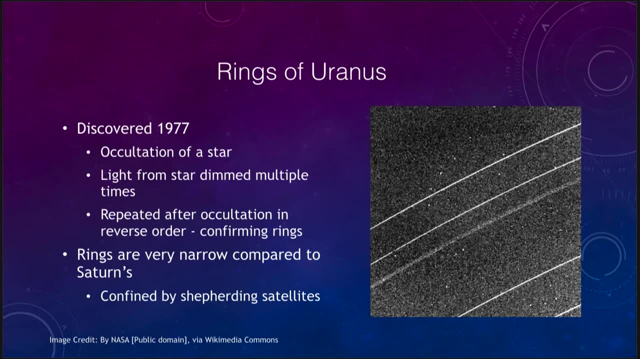 And other times they would be pushed apart. Now Saturn again has the primary and most detailed rings, But the other objects have rings as well. So let's look at Uranus here. Uranus's rings were discovered in 1977. A couple of years before Jupiter's were discovered. 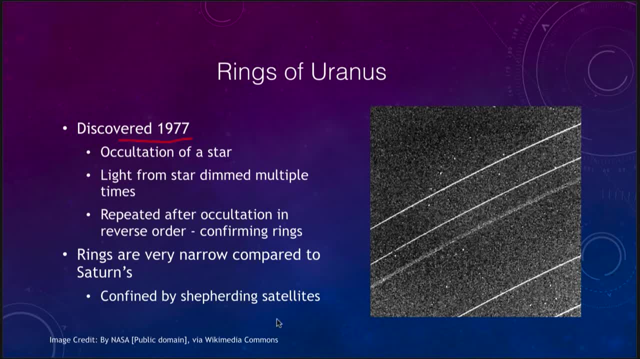 Although hundreds of years after the rings of Saturn were known, They were discovered during the occultation of a star. What happened was Uranus was going to pass in front of a star, So astronomers wanted to study how its light dimmed As it passed in front of the star. 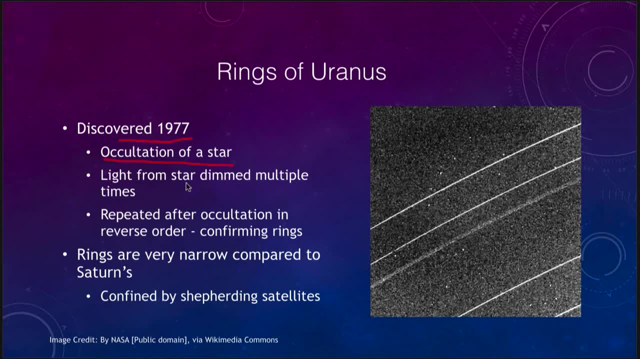 But before the planet passed in front of the star, We saw that the light dimmed multiple times And this repeated after the occultation, in the reverse order, Kind of confirming that the rings did exist. So the rings as the star was passing. 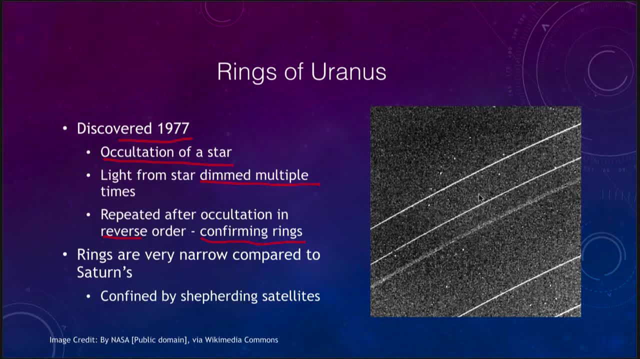 The rings would pass in front of the star And that would dim the light a little bit As each of these rings passed in front of the star in turn. And then you can imagine on the other side You went the other direction And it would pass through the rings in the opposite order. 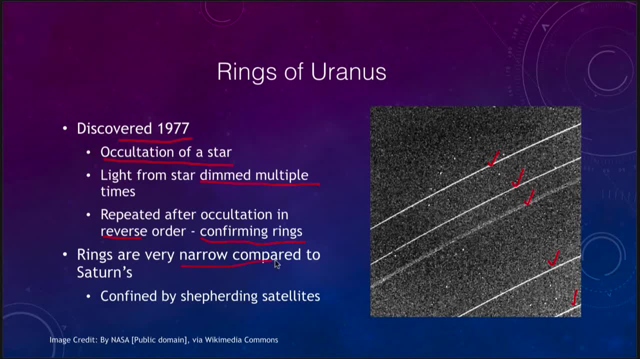 Rings are extremely narrow compared to the rings of Saturn, So we see the rings of Uranus here very, very thin. These are not the wide, broad rings that we saw of Saturn. They are actually confined by shepherding Saturn. They are little satellites. 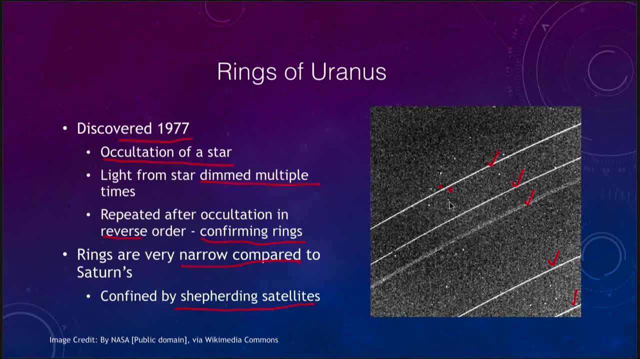 Little moons that will orbit just on one side And just on the other side And keep all those particles in line. So, essentially, as one moon orbits And the other moon orbits, Their gravity will keep those very well confined. Now, what is the composition of these rings? 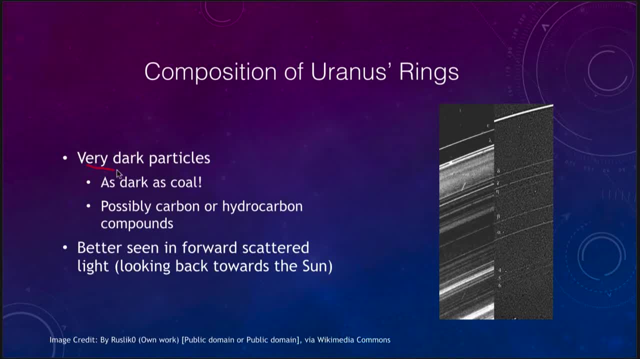 Well, they are very dark particles Again. why do we not see them from Earth? They are not icy Like the rings of Saturn. They are in fact as dark as coal. So we don't really see them in forward, Looking forward. We do see them in forward, scattered light. 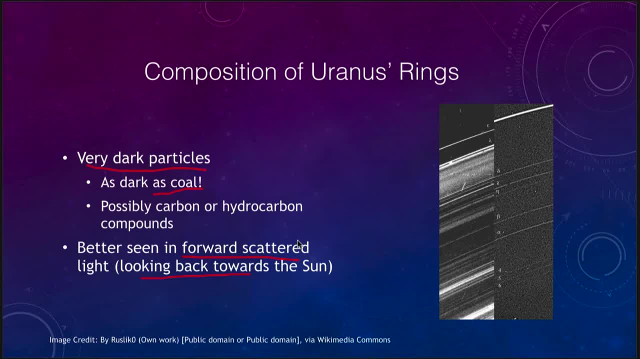 Which means we are looking back towards the sun. So if we look at the image here, There is what we see of the rings from the Earth. But if we were behind them, Looking back, we would see all sorts of light scattering through these rings. 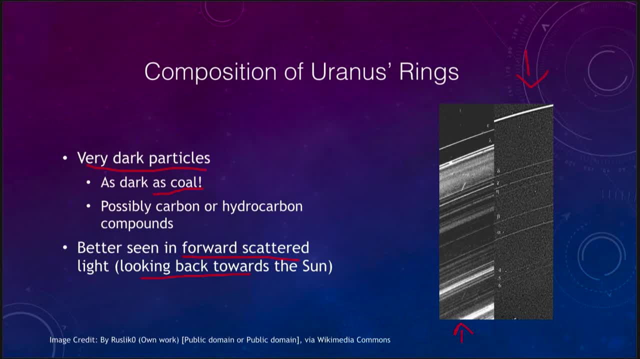 So there are a lot more structures there That we don't actually see From Earth But that we had to get around behind, And the only object that really went close to this Was the Voyager 2 spacecraft That actually went past Uranus. 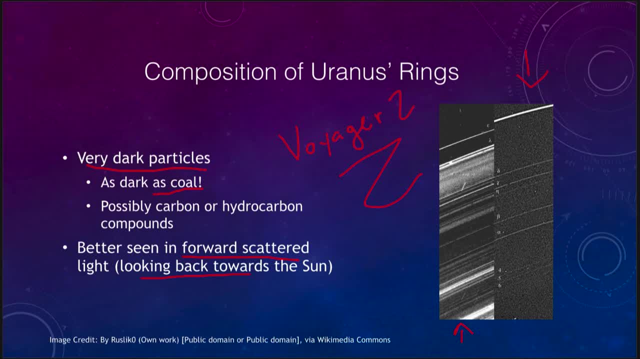 And was able to turn back And look back to the sun. But it is a very different structure you get If you are looking from the sun Versus if you are looking from behind. When you look from behind, Other than the composition we know is different, 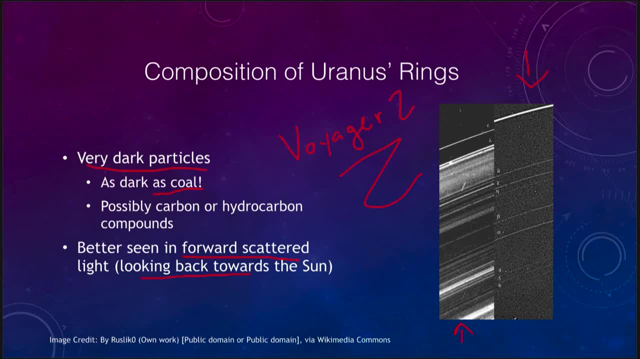 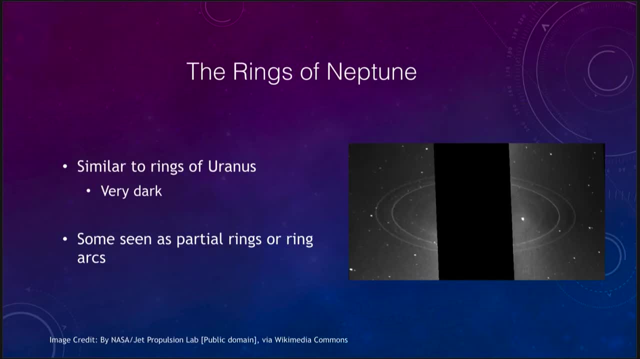 We see very similar structures To what we saw on Saturn. Now, the last of the objects to look at with rings Would be Neptune. Neptune has very, very dark rings, In many ways similar to those of Uranus, And they are quite dark. 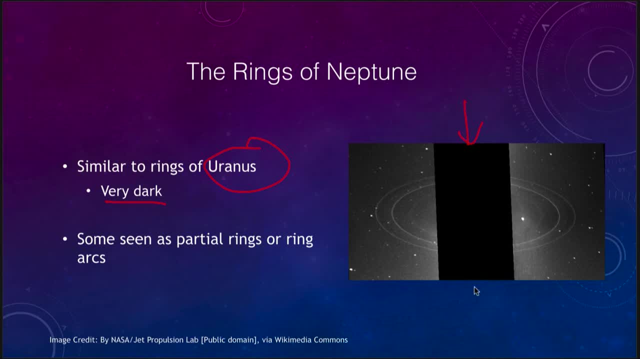 And we can see them here. This is blocking out the light from the planet, Which would overwhelm the very faint rings. So they are there, But we have to block out the planets light In order to even be able to see them. They are seen as arcs sometimes. 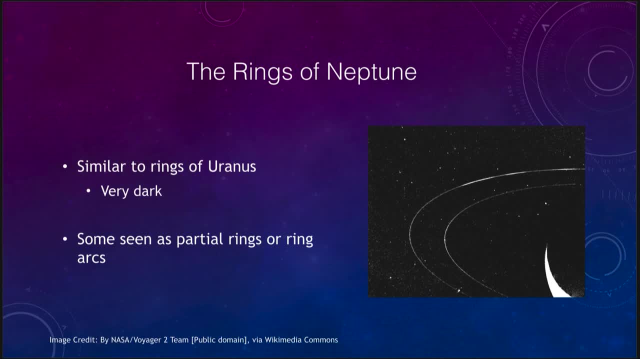 So if we look here, Another image of it, And we see that there are denser areas Of the rings And there are areas where there is less ring material, So, unlike the rings of Saturn and Uranus, Which seem to be relatively smooth, 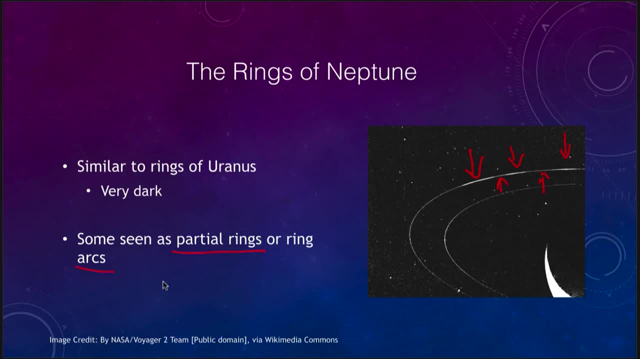 The rings of Neptune are sometimes seen as partial rings Or even just ring arcs, So there is a little bit of a difference there in Neptune. Are these relatively young or relatively old rings, Something we really do not know. Now, the last thing we want to look at: 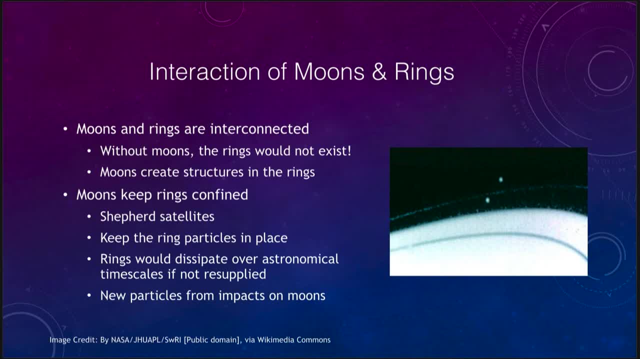 Is the interactions between the moons and the rings. There is an interconnection between these And, in fact, without the moons The rings would not exist. Where did the rings come from? Probably from particles blasted off the moons in impacts, And that would then give the rings 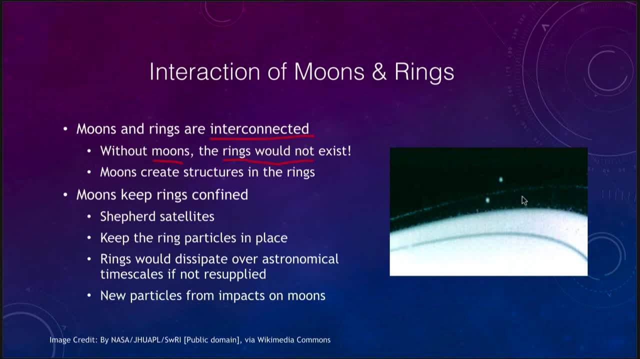 Particles a supply of material. The moons also keep the rings confined, And that is what we call the shepherding satellites Which we see here orbiting around And keeping the ring particles in this very narrow ring Well confined. So they keep the ring particles in place. 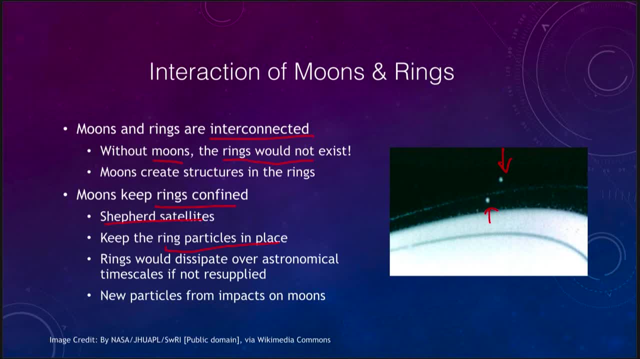 The rings would dissipate over astronomical time scales. If we run models of all these particles orbiting, We would find that they would slowly dissipate Out into space. There has to be some form of resupply, And that would be from the moons. 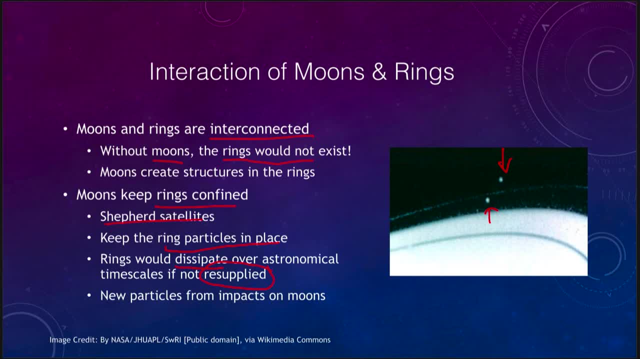 That impacts on the moons Could actually throw more material back into them And replenish the ring particles. So where do we get those new particles From? impacts on the moons. The moons also create all of the structure We see in the rings. 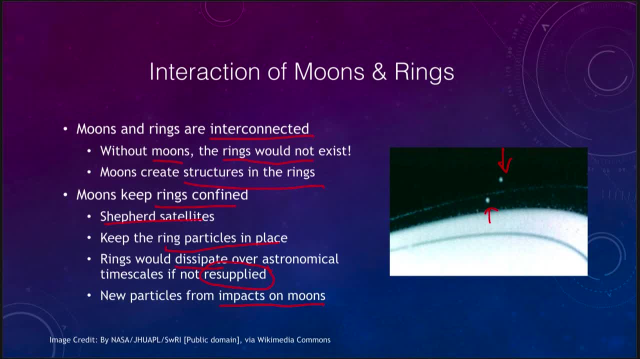 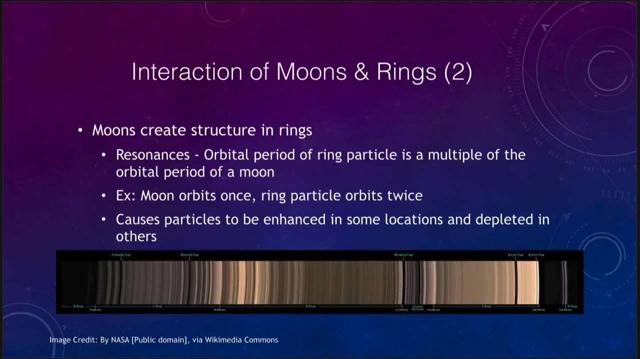 The rings would be much smoother without the moons. But the structures that we see are Different patterns that we see, And if we look real close at one of the rings here, We can see all sorts of structures That are present in the rings of Saturn.